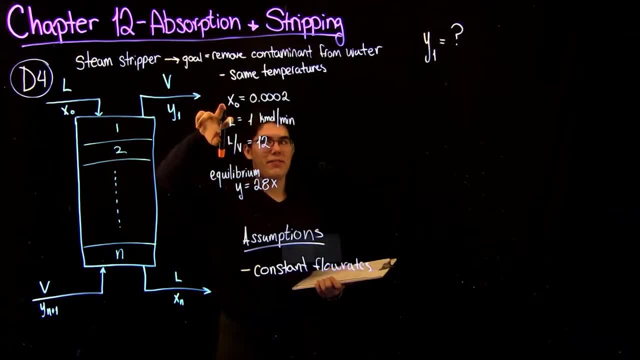 And we can actually make this assumption because, as you can see, it's a very, very dilute system with small compositions. So that means that this component, moving from the liquid to the vapor or the other way around, isn't really going to change the overall flow rate. 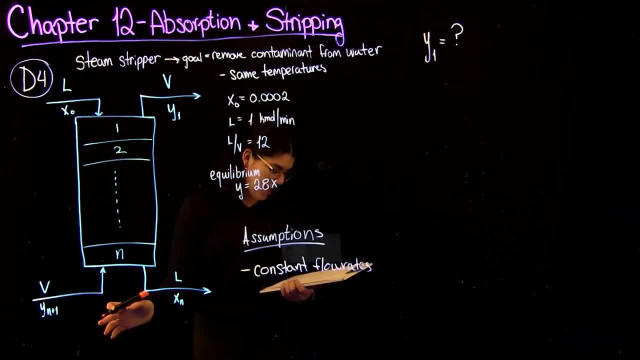 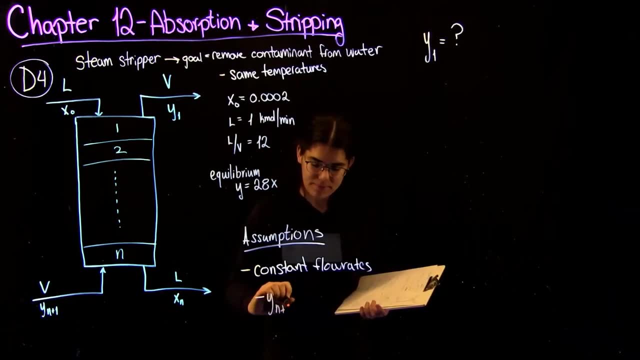 Another assumption we're going to make is that the entering steam or vapor coming in is pure, or that Yn plus one is equal to zero, Just because that wasn't particularly specified anywhere. But it's a safe assumption to make because we know it is a steam stripper. 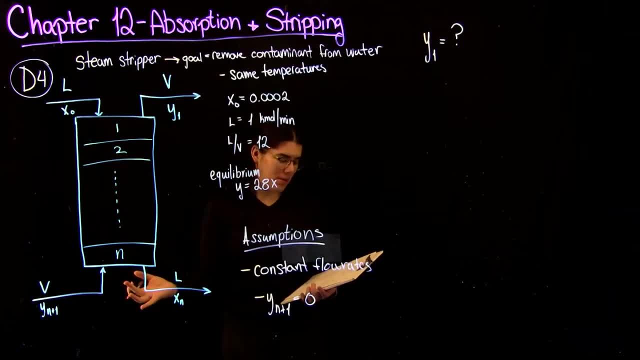 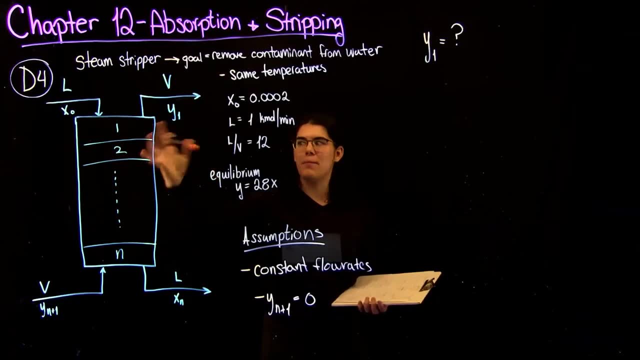 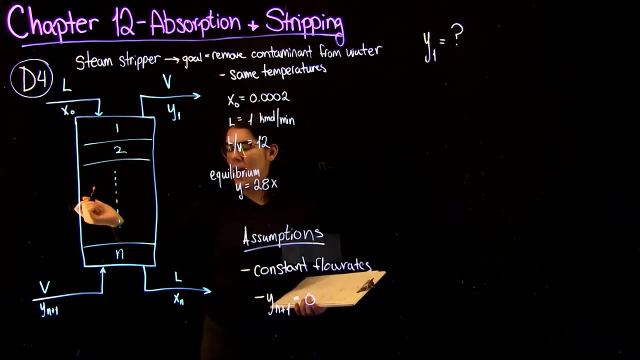 So we can assume we would like the steam coming in to be pure. OK, so the first question asks us to find the value of Y1. And we're going to be able to do this by deriving our operating line for the system. So, like we always do, our operating line is just going to be a mass balance. 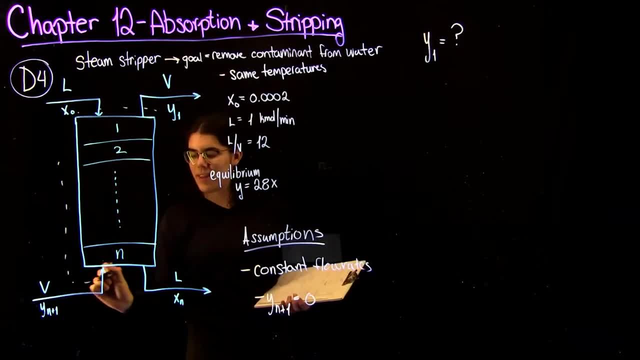 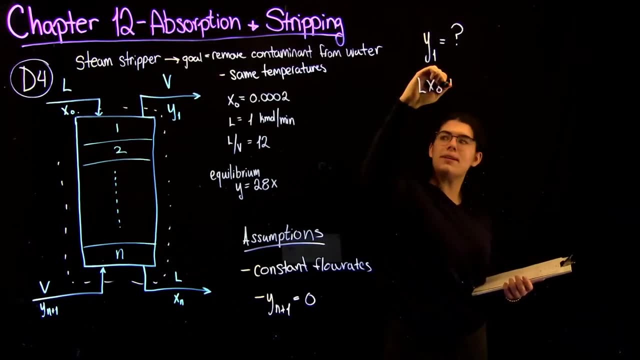 And for this case we're going to do it just around the entire system. OK, so what that looks like is Lx0 plus Vyn plus one, So that's what's going in is going to equal what's going out, So that's Vy1 plus Lxn. 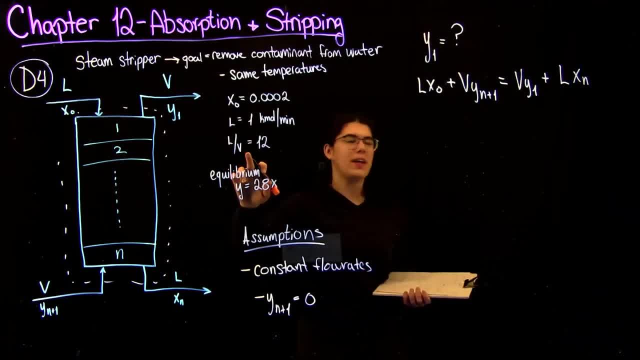 And since we're given the L over V, we can solve for Y1 one of two ways We can find V, or we can put this into the form of our operating line And since we're going to need the operating line later to find the total number of stages, 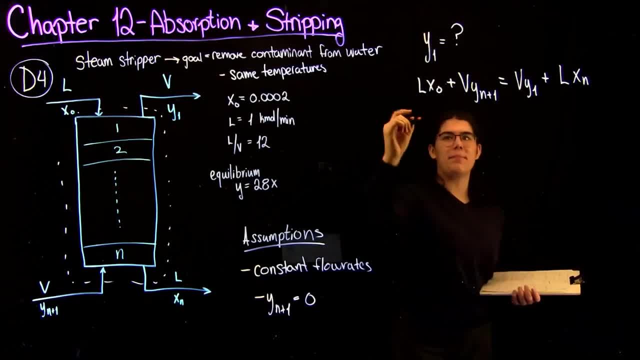 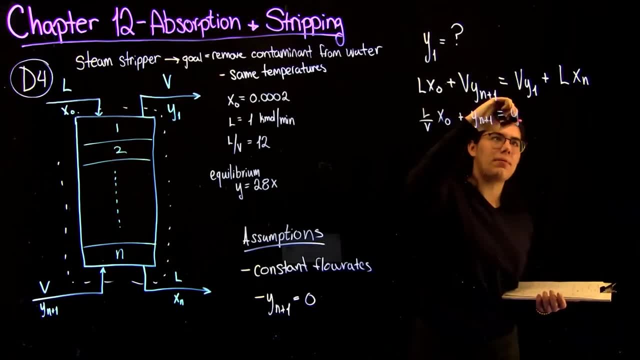 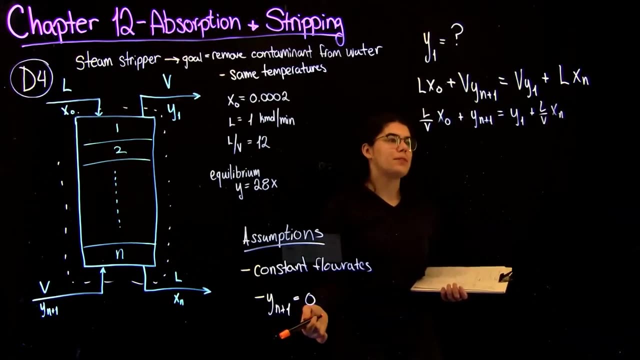 we might as well just do that now. So if we divide everything by V, we get L over Vx0 plus Yn plus one equals Y1 plus L over Vxn. Since one of our assumptions is that Yn plus one equals zero, we can just cross that off. 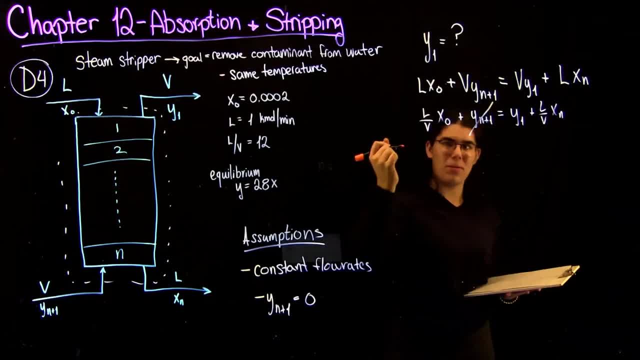 And we can just rearrange this to get it into a useful form for us. So we're going to get Y1 equals L over Vx0 minus xn. Or to get the operating line equation form, we'll just plug in the numbers that we know. 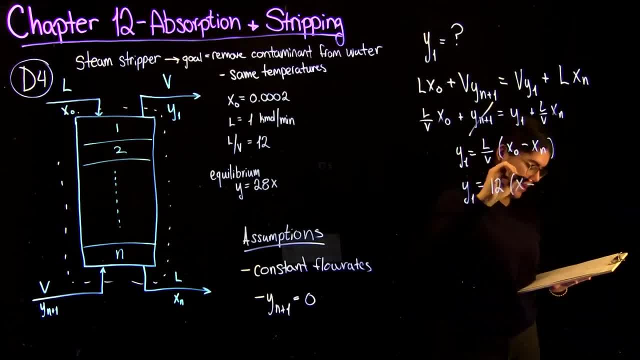 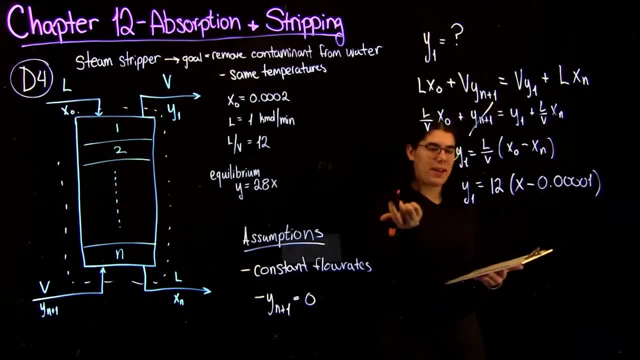 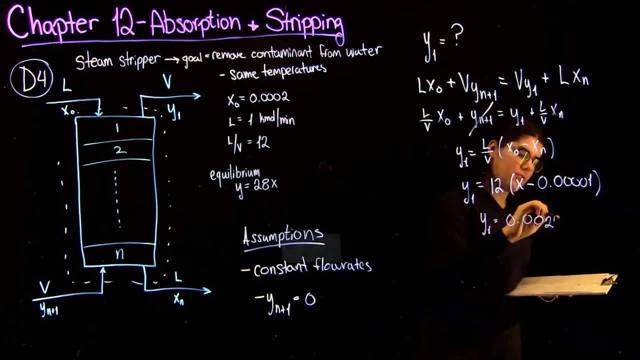 So equals 12x minus. and then the composition of xn that was given. OK, so if you just plug in your known values, you're going to get that Y1 equals 0.00228.. OK, so, like I said, this is a dilute system. 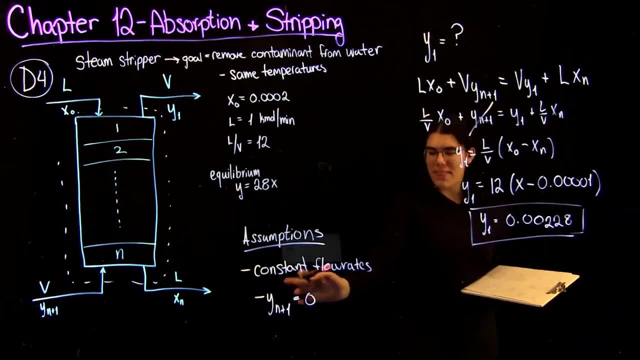 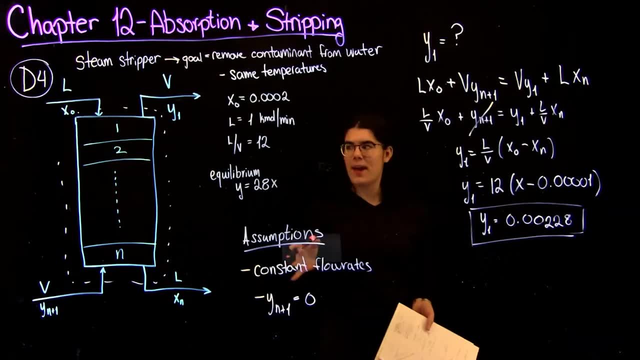 So it should be a really small number And it kind of just confirms that our assumption of constant flow rates was OK for this case. OK, so to find the number of stages, you're going to do a McCabe-Thiel diagram, just like you do for a distillation column. 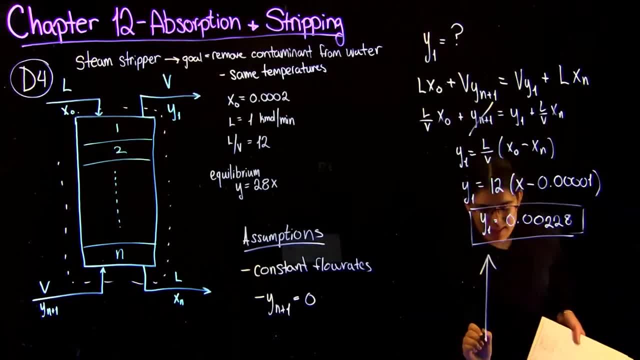 The only difference is that now it's going to be two straight lines as opposed to a curvy equilibrium line. So because we're doing, If you have a steam stripper here, your equilibrium line is going to actually be on top. So when you plot it, you'll see that it's going to look like this: 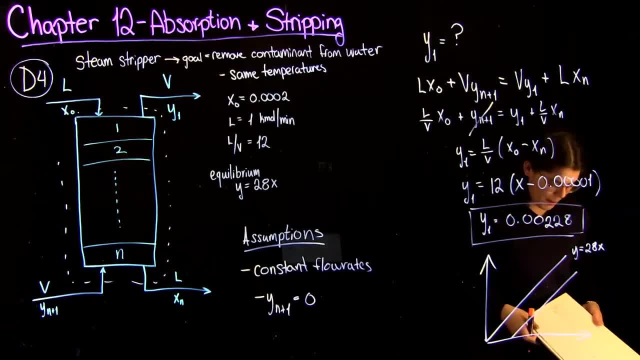 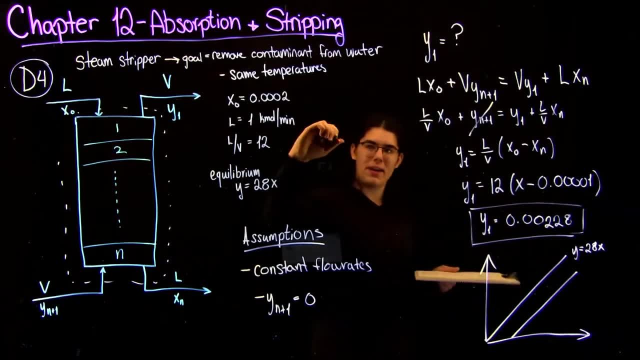 So you're going to have your equilibrium line here and you're going to have your operating line down here. The two most important points you need to plot your operating line in this case are going to be- I'll write it over here- Your xn comma yn plus 1 and your x0- y1.. 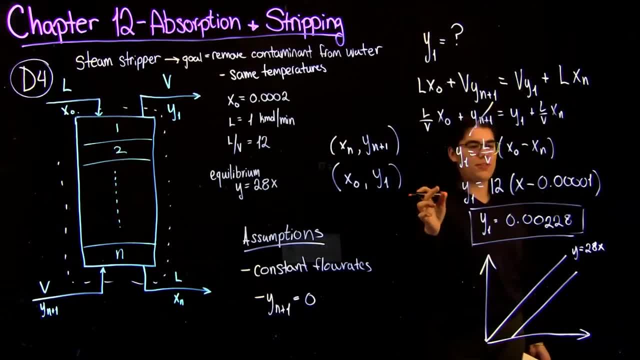 And if you just use these two points to construct the line- or you can also do it using this equation- You have both, but I find it's usually easier just to connect two known points on a graph- You'll be able to set this up, and you're going to find that you need three stages to get what you need. 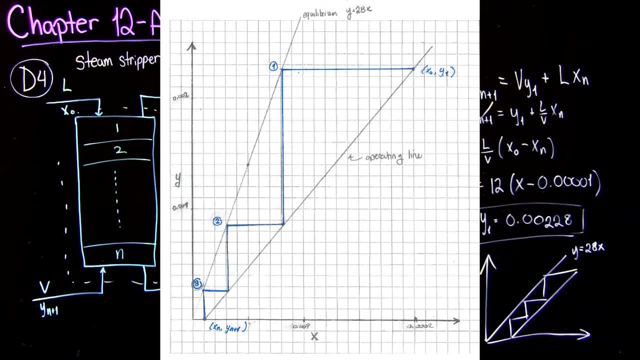